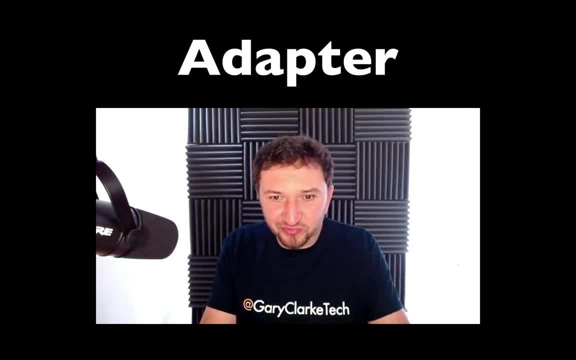 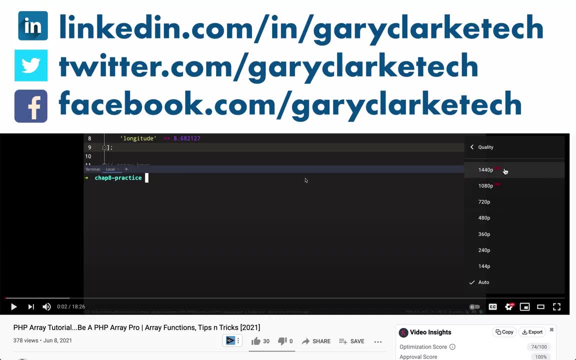 socket. So in this one we're going to look for that kind of problem in our code and we're going to solve it using the adapter pattern. Some housekeeping first. Choose high definition for the best viewing experience and if you would like to join a growing group of software developers, 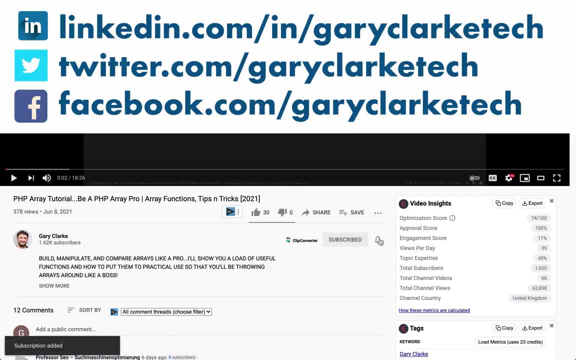 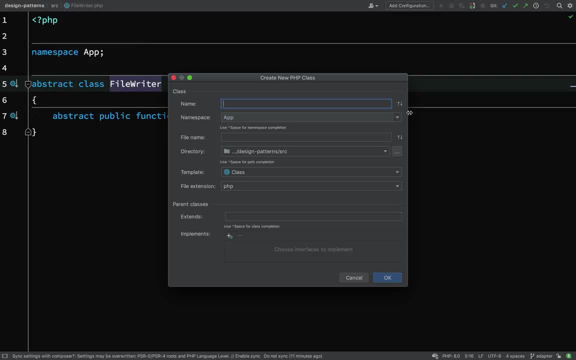 and take your skills to a new level. all you need to do is subscribe and click the little notification icon and welcome First example. we'll go back to our file writer, which we created in the dependency injection lesson, and let's imagine that there's been an office vote and 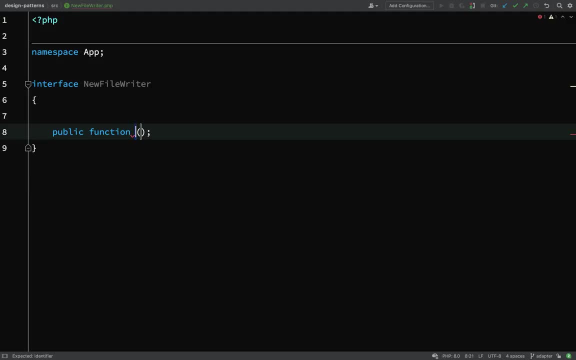 we've decided to use a new package which has a new file writer interface and we're going to build into this some differences from the original file writer So that had a method called write to file which returned a boolean. This one is going to be a little bit more complicated. We're going to 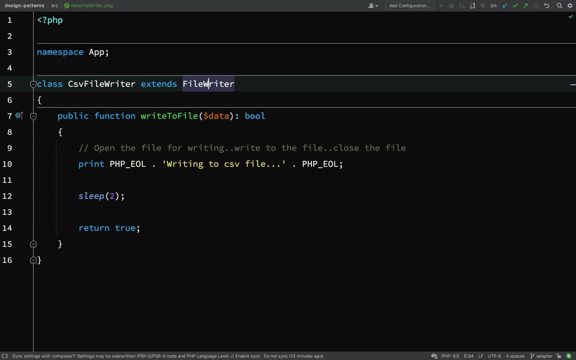 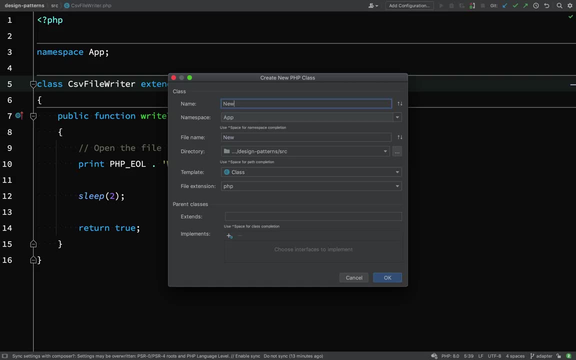 have a method called write which won't return anything. It just writes to the file. Nothing is returned. So start thinking about the code we've already written. By that I mean the client code of the file writers which are calling a method called write to file. It's going to be incompatible. 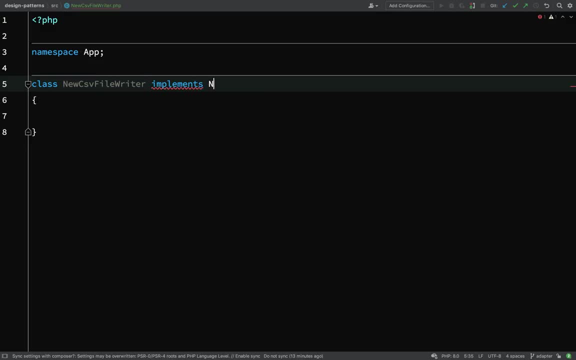 with our new package. Let's write a class which implements a new file writer. So, like we have the CSV file writer, we'll now have a new CSV file writer. We'll go and borrow a bit of code from the CSV file writer. We'll go and borrow a bit of code from the CSV file writer. We'll go and borrow. 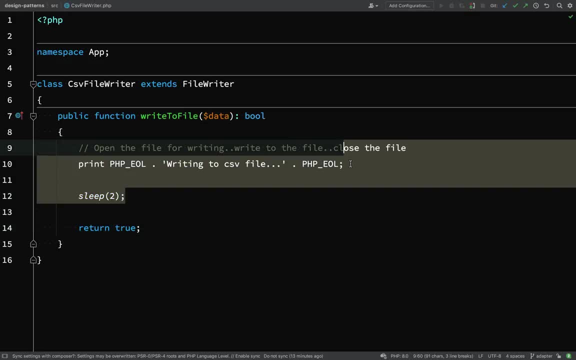 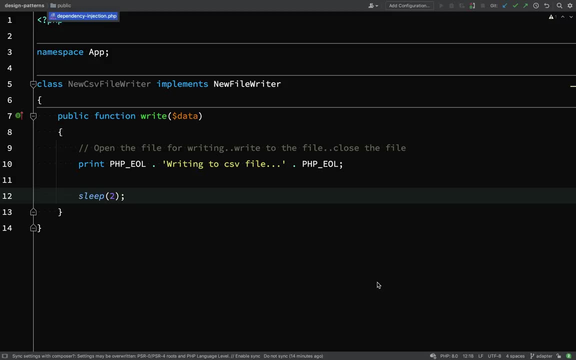 a bit of code from the CSV file writer. We'll just take these top two lines, because of course we're not going to return the boolean in our new method. I'm going to go and create a file where we can test some of this stuff out. So, inside of public, I'll create just a new plain PHP file. 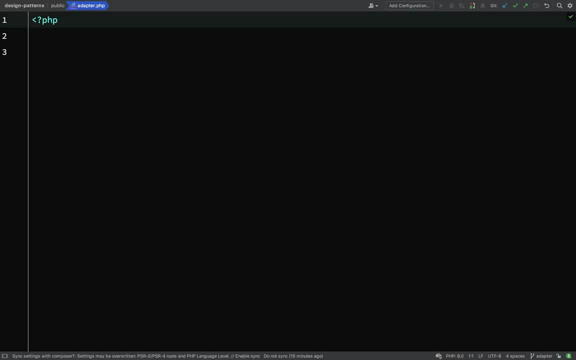 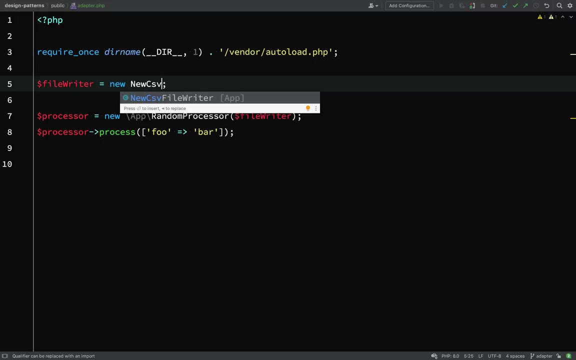 and I call it adapter. Okay, so let's start off with some code that we've used before. We can borrow some of this from the dependency injectionphp file, and there we're just requiring the vendor autoload, and instead of newing up a JSON file writer, we're going to create a new CSV file writer. 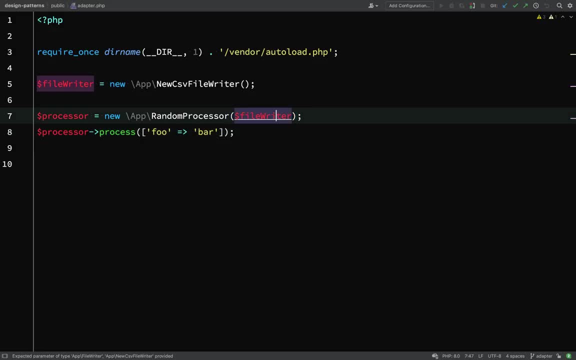 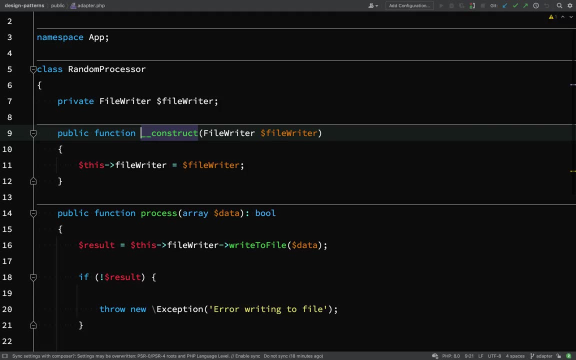 If you look at the random processor, which is the client code that's going to use this, we have a problem. Expected parameter of type: app: file writer. app- new CSV file writer. provided Let's look at the random processor. So, as you can see, here in the constructor, we're expecting a file writer. However, 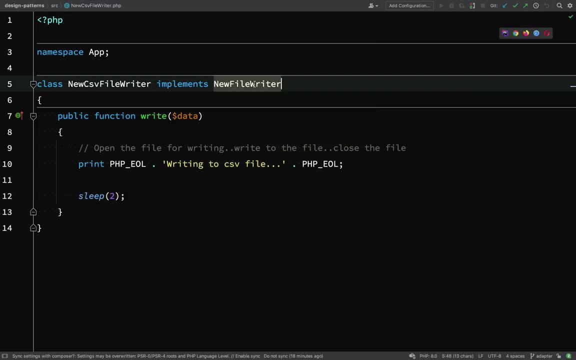 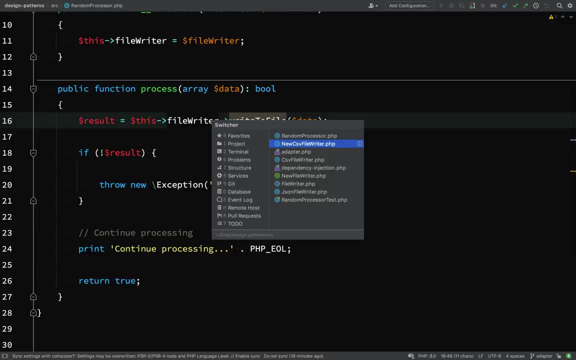 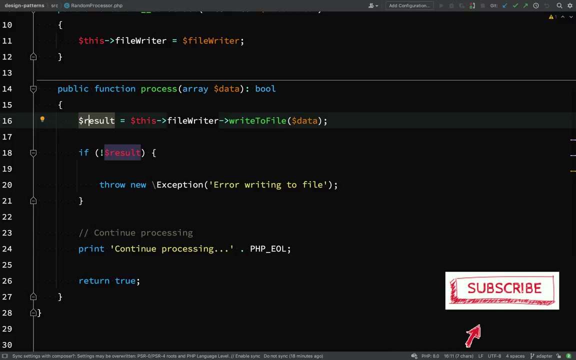 our new CSV file writer is going to be a new CSV file writer, So let's look at the random processor. implement new file writer, incompatible. Also, we're expecting the file writer to have a method called write to file. Our new file writer has a method called write. Thirdly, we're expecting that 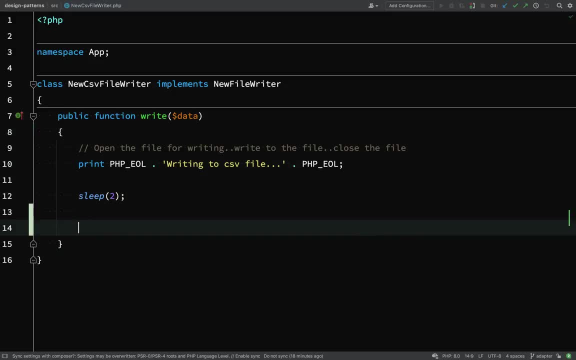 method to return a result, but our new package, the write method, does not return anything. So I'll just mark this as void, just to be explicit and fix: the typo does not return anything. So presently our new package, our new code isn't going to work. We need to write an adapter and this: 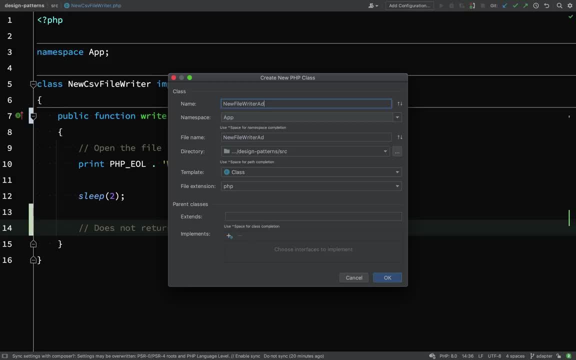 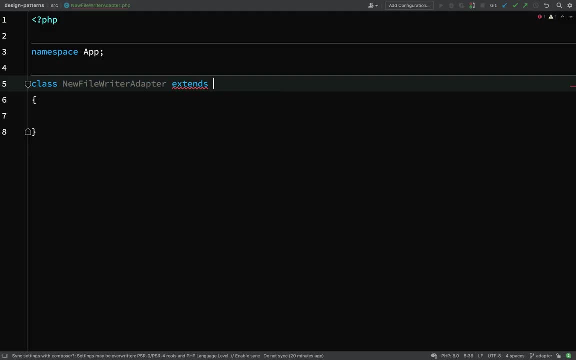 is how we do it, So we'll call it new file writer adapter, because the new file writer is a class or the interface which is going to be adapted to work with our existing client code, And the way it works is this: We extend or implement the class or interface that your client code is using and you 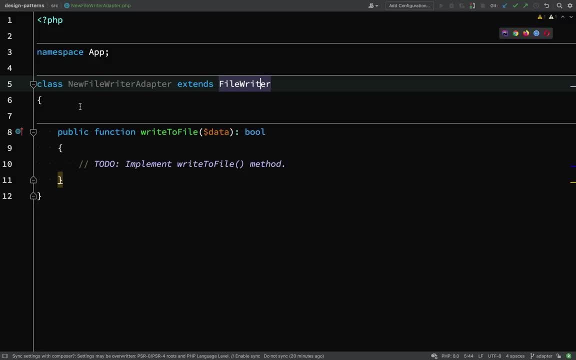 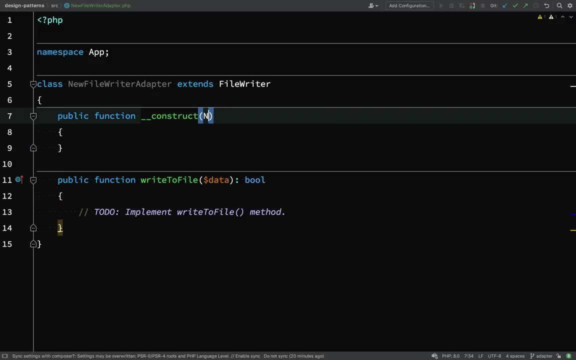 inject the class or interface that your client code is using and you inject the class or interface that needs to be adapted. So in our case, we are extending the file writer, that's existing file writer and what our client code is currently using. And then I've created a constructor and I'm 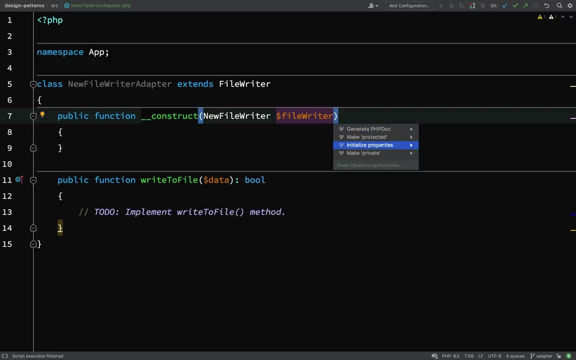 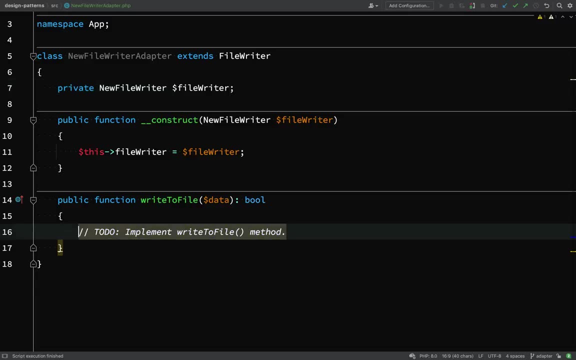 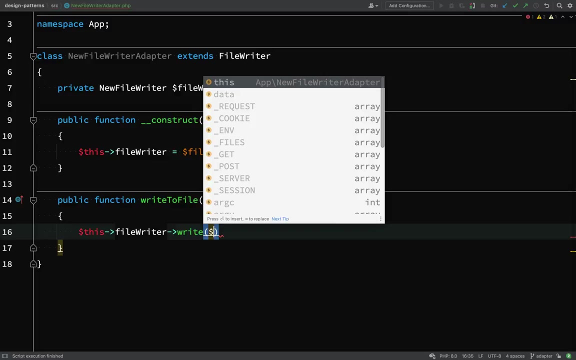 injecting the new file writer through the constructor. I'll initialize the properties and then we need to put something in our write to file method in order to write to a file using our new file writer. So we can say this: write, because write is the method. on the new file writer, We pass in the data and in order to stay, 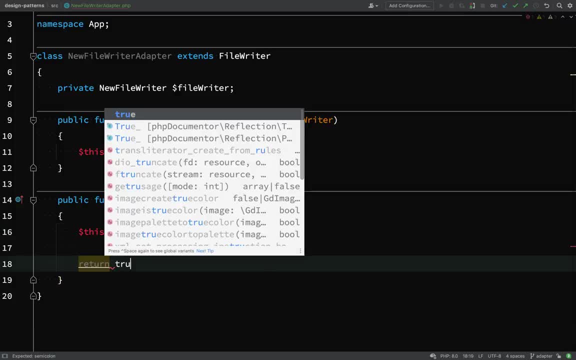 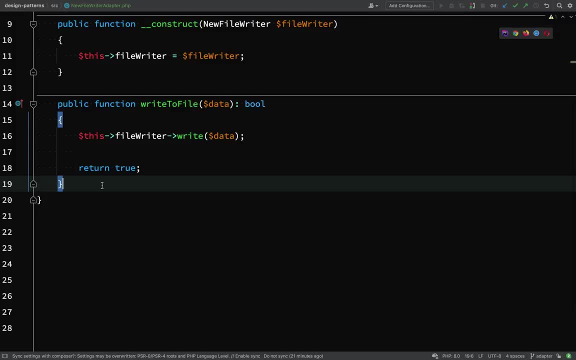 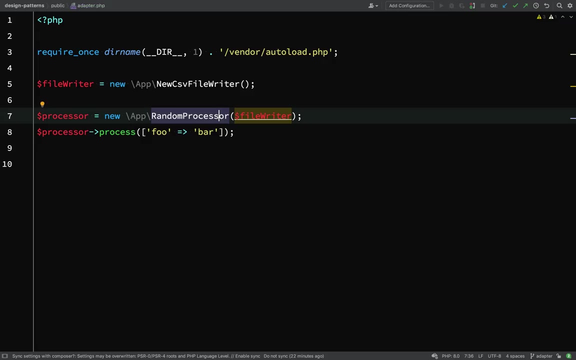 true and compatible to our current interface. we need to return a boolean, So let's just return true from there. So have a look at what we've done. We've got a method which is compatible with our current interface, but we're still able to use the functionality of the new package. Let's go. 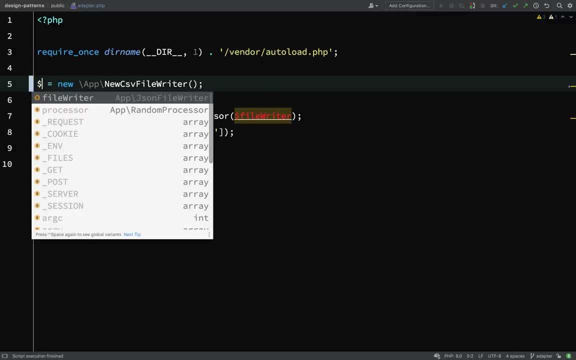 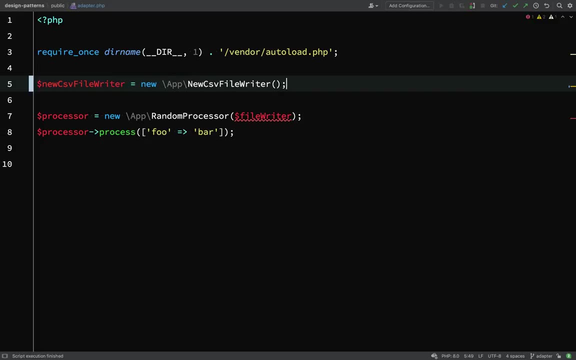 over to our adapterphp file and change this now to use the new file writer. So we've got a method to use our new code. So we're going to say new csv file writer equals new csv file writer, and then what we need to do is then inject that into an adapter. So file writer equals new new file writer.